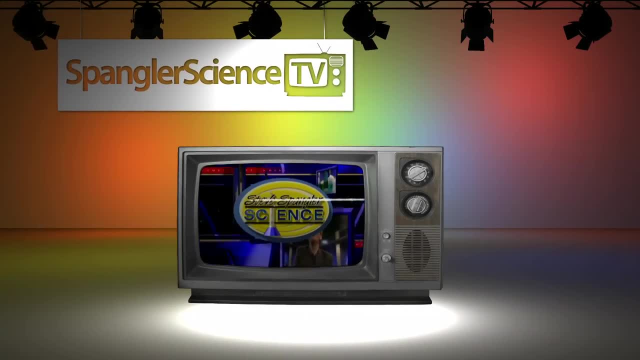 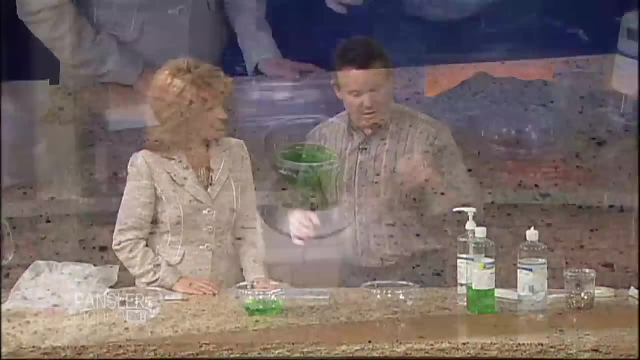 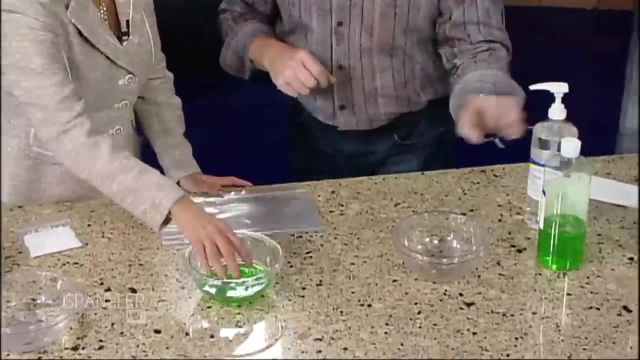 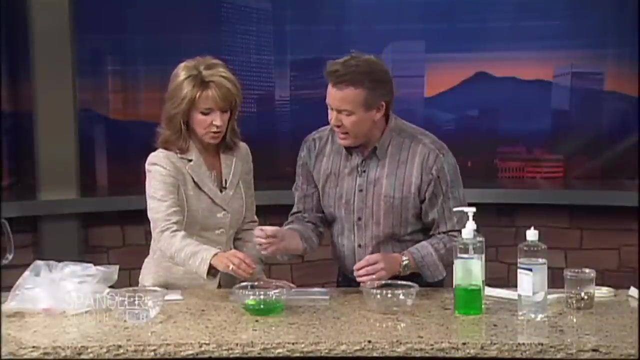 I want to show you kind of the best slime, I think, And it's made with something called polyvinyl alcohol. It's actually a liquid that you see here. It's a polymer, meaning it's a long chain of molecules. Go ahead and put your fingers down inside. No, not that. No, it's okay, It's fine. It is goopy, isn't it See? Yeah, just a little All right. So when you feel it like this but it doesn't stick, like you can't pick up the whole thing, right? No, because they are long strains of molecules. So 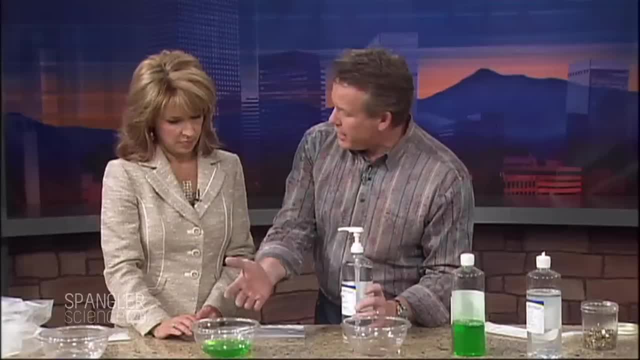 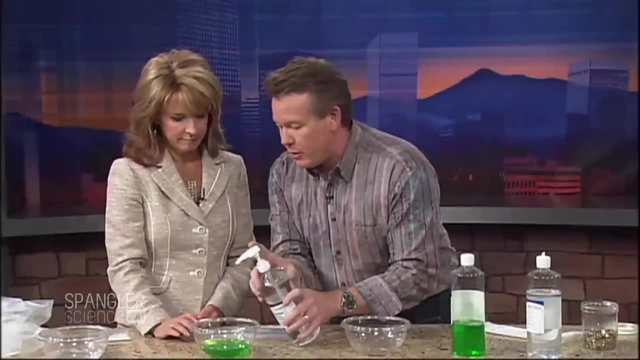 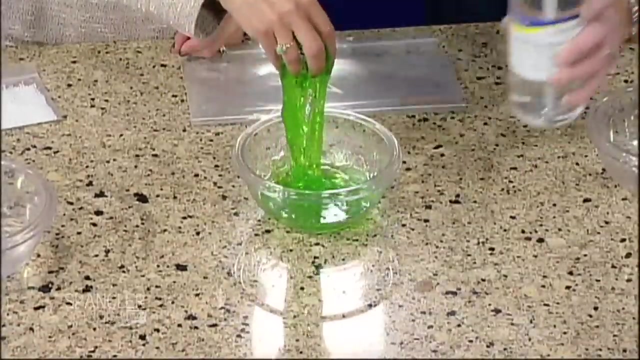 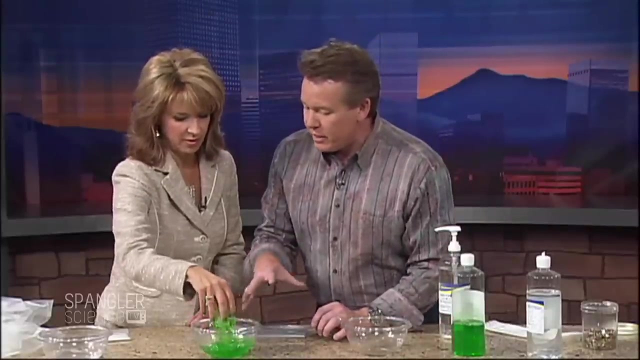 what we do is we add to this mixture right here- and you can do the same thing with, like, Elmer's glue and a little bit of water- We're using borax. So borax is a soap, and those borax molecules link it together. So here, watch this, Get your hand down inside. I'm going to squirt this in there and now squeeze it around. Oh, now you got slime. Can you tell immediately? There you go, Now mix it in there. Isn't that great, Yeah, Oh yeah. You see, You just keep playing and I'm going to show you that this is a little easier to come up with and there's a little bit more connection than you could ever imagine. I'm going to reach underneath you like this. 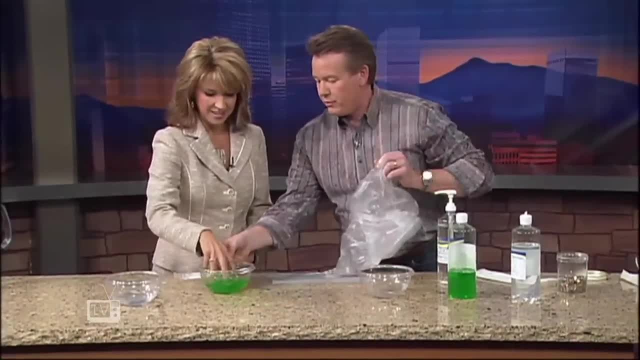 got it, This bag, because I know your hands are a little goopy. It's okay, Keep them there, You're just fine, Keep playing This bag. here is actually this material, right, But it's in its clear form. 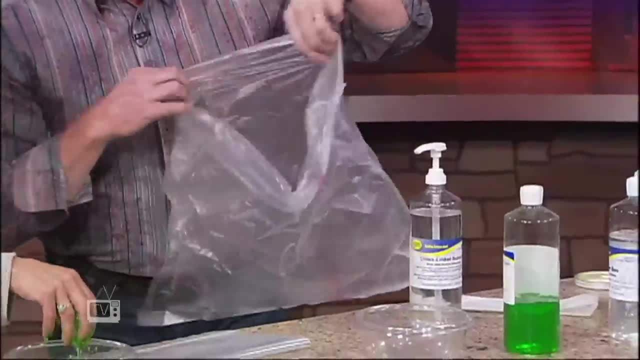 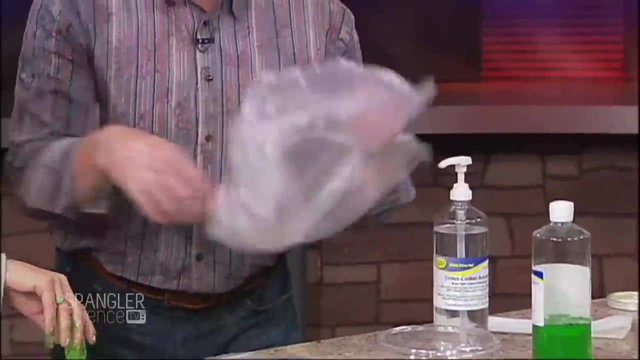 This is a bag made out of polyvinyl alcohol. They use these in a hospital setting when they want to put sheets or something in there that they don't want other people touching. They will close this up and literally just put it in water, And so watch what happens. I'm going to use this in a 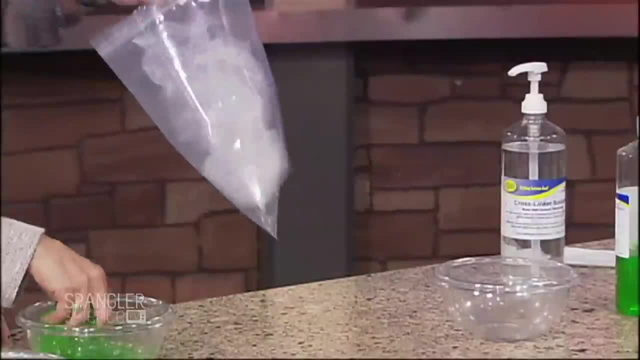 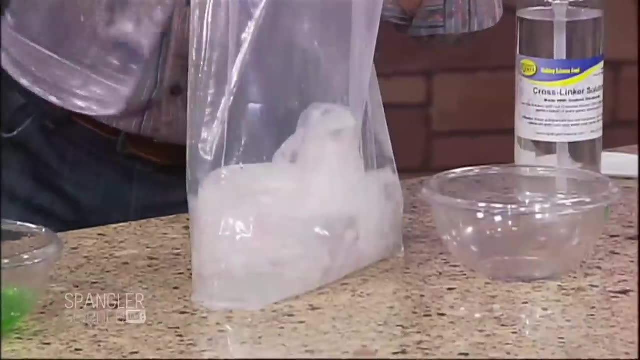 Ziploc bag and I'm going to reach just around you like this and grab this. I didn't expect that I'd make your hands that dirty all the time. Look at this. This is just water that goes down inside, like this, and this bag literally. 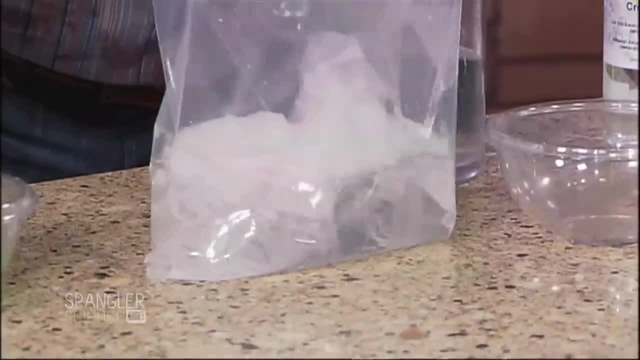 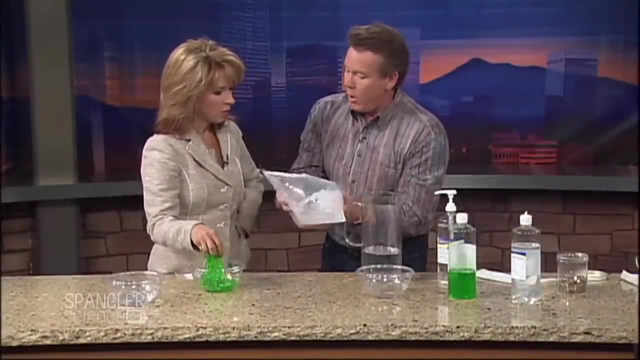 dissolves in the water. So if you can get your hand on one of the bags- for example, maybe a nurse or hospital, something like that- this bag dissolves. So they literally just throw the bag in the wash machine and it dissolves, washes out and nobody had to touch the sheets. So when 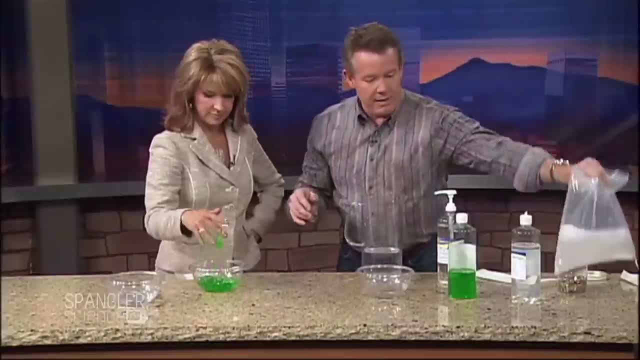 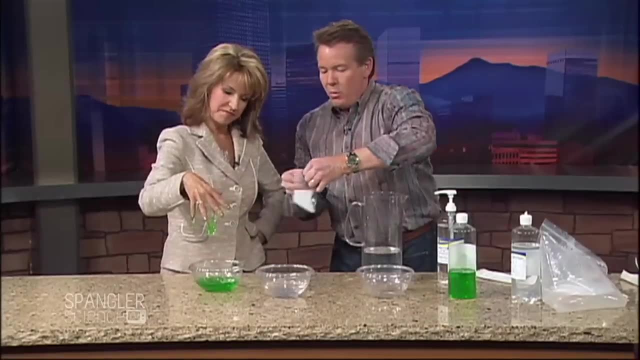 we're learning. we always try to connect something like this to something that may be a little bit more meaningful for kids or something that they'll remember. Doesn't that look great? Look at this. I've got a mix-in for you: Slime.